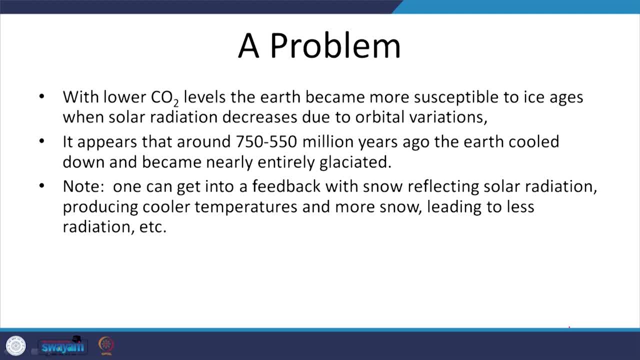 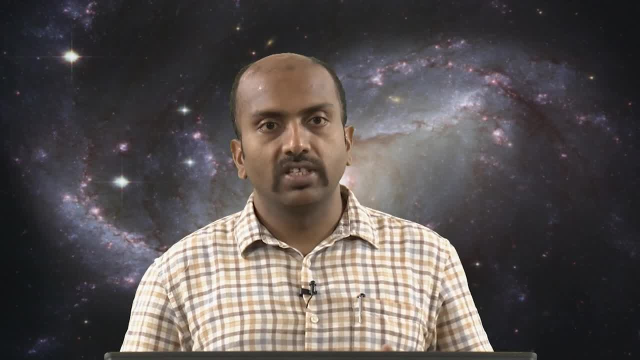 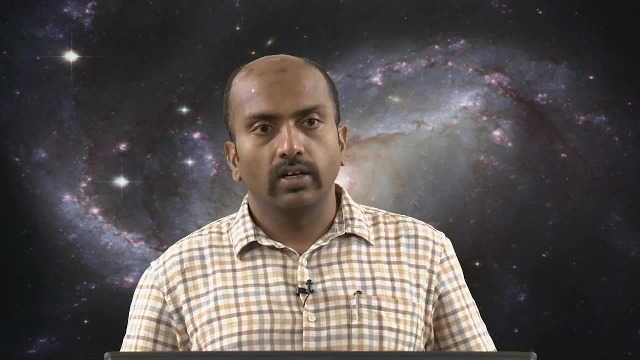 which was basically the volcanic eruptions. Volcanic eruptions have created a lot of CO2.. We have seen how CO2, how much CO2 was there in the system and how this CO2 was lost into the system, into the Earth itself, and right now we do not have much CO2. 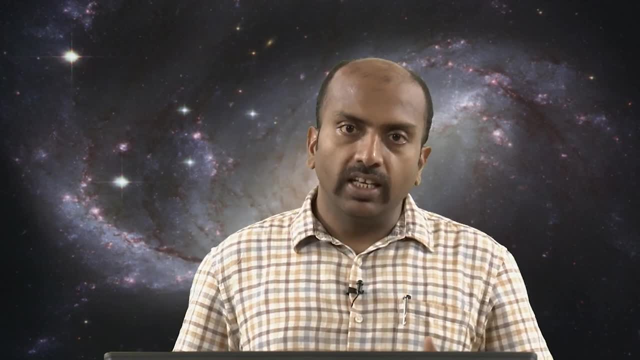 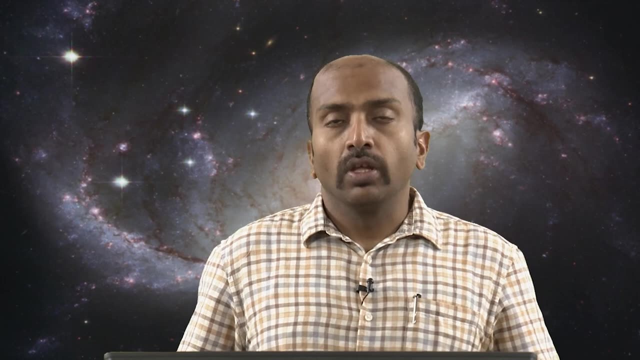 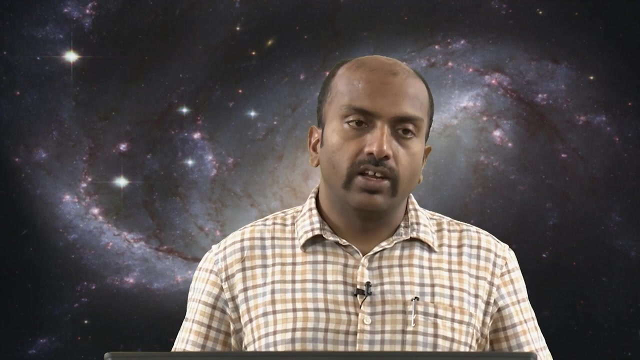 in the Earth's atmosphere. ok, So with the decreasing levels of CO2 on the Earth, Earth became more susceptible to ice ages. Let us say CO2 is a very important species because it has the tendency to be excited by the infrared radiation bands. That means 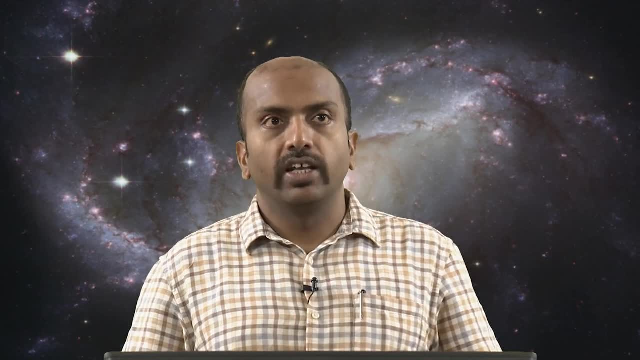 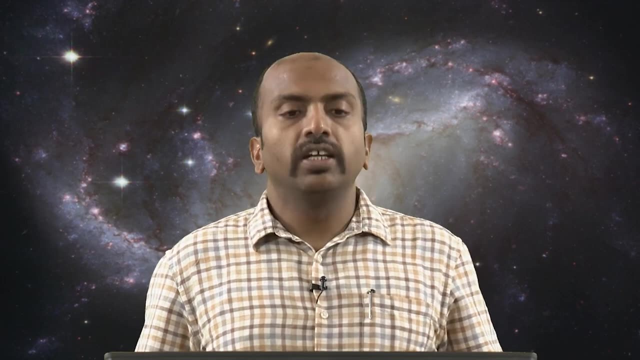 that it has the ability to trap the outgoing infrared radiation In the heat is generally given a term as infrared radiation. infrared radiation is heat, So CO2 has the ability to keep a planet warm. So if you do not have CO2, that means 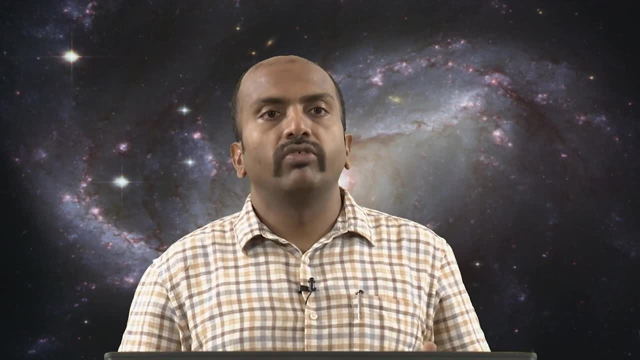 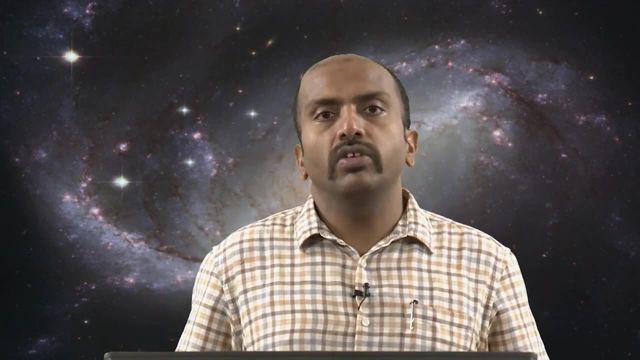 that you will. the planetary surface will be hot when it is exposed to sun, when it is a day time and when you have the night time, the planetary surface will be very, very cold. That means the average temperatures between the day and night will fluctuate. 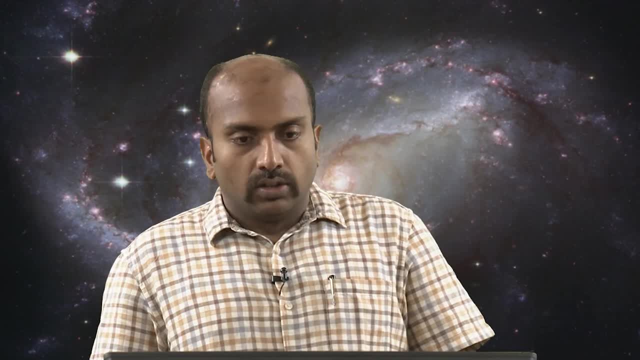 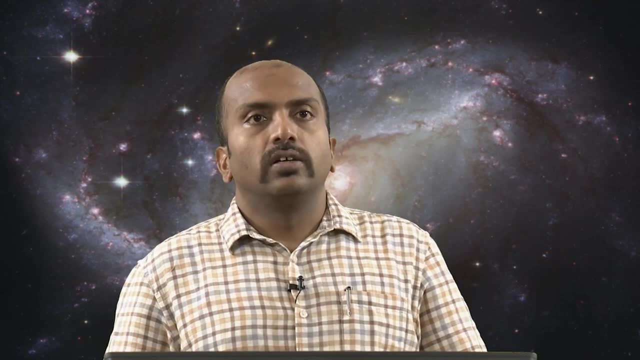 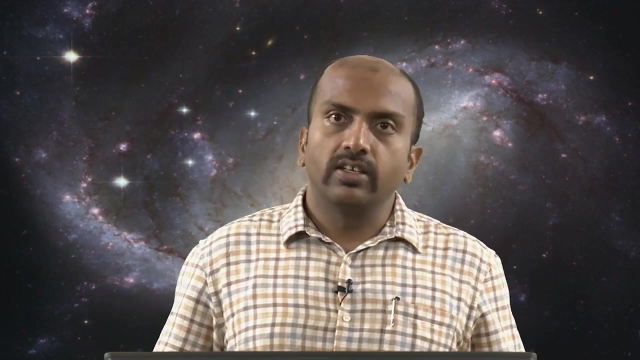 over a very large band. So CO2 is a very important species just because it can hold the heat and it can maintain average temperature which is not very different from day to night. ok, So CO2 levels were decreasing due to the photosynthesis reaction which was happening. 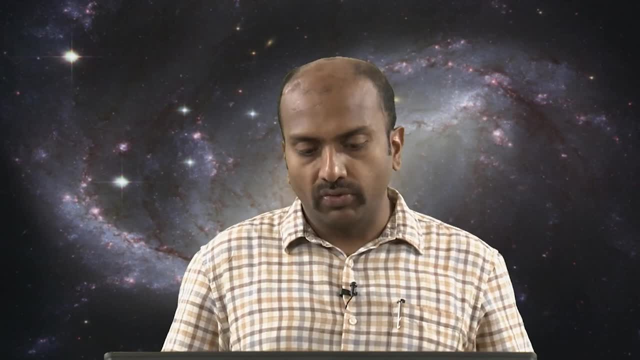 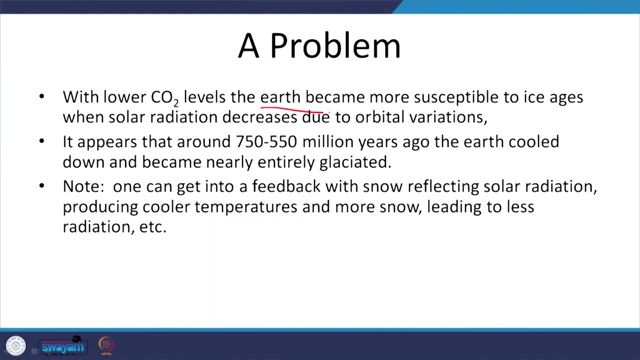 for a at a very fast rate, building up a lot of oxygen in the atmosphere, right. So, with the lower levels of CO2,, with the decreasing levels of CO2, the Earth became more susceptible to ice ages, because the temperatures were going down when and when the solar radiation decreases. 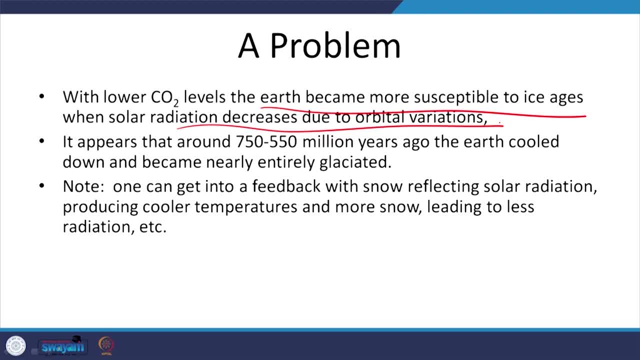 due to the orbital variations. ok, Now it appears that nearly 700 to 550 million years ago, the Earth cooled down and became nearly entirely glaciated. So it happened once. I mean the ice age was there for a reason, with the decreasing levels of CO2.. 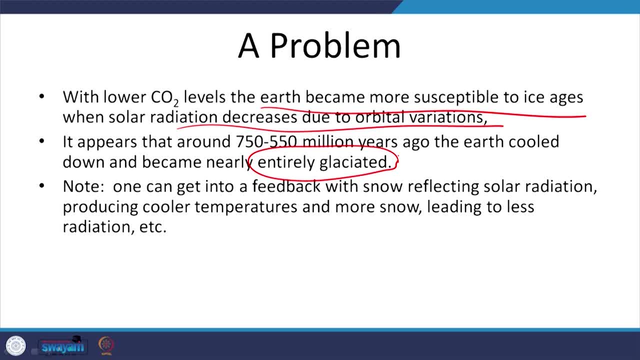 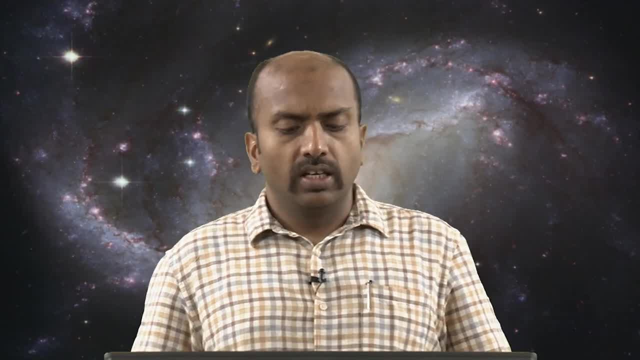 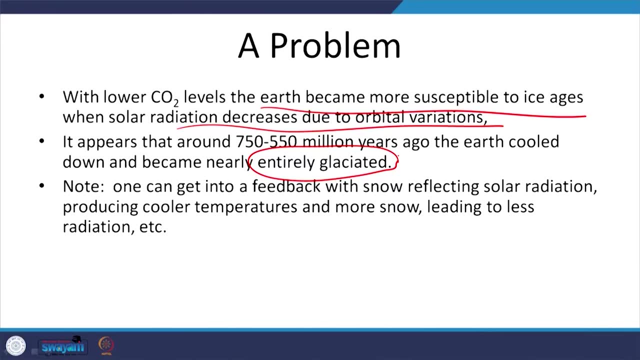 Nearly 550 to 750 million years ago, the Earth has cooled enough so that it was nearly an ice age. the entire Earth became nearly glaciated, So it may be possible that how did we got out of this problem? So here, it is a very important point to know that. 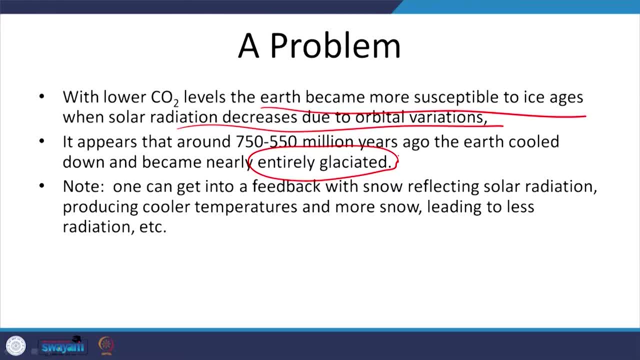 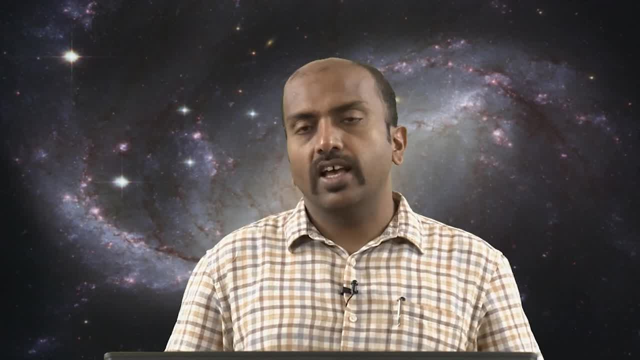 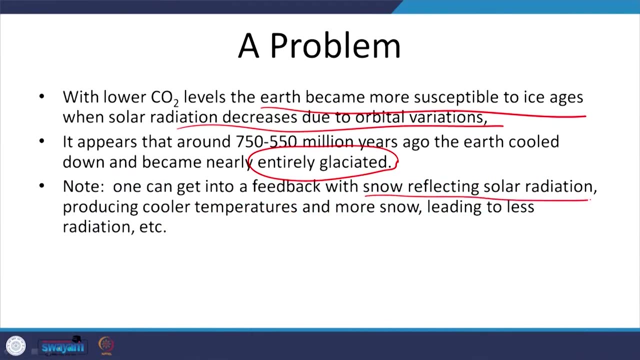 when the ice cover of on the planet increases, what happens? due to the high reflectance of the of the ice, that means ice has the ability to reflect most of the incoming solar radiation that falls on it. So snow reflecting snow can reflect large amounts of solar radiation. 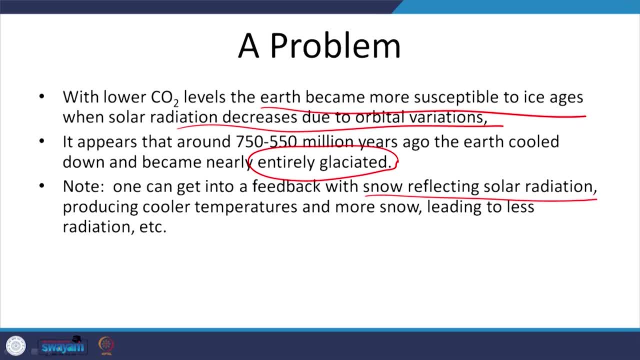 that means once the ice formed there is, even the solar radiation is reflected more. that means you go into a negative feedback in which the more and with time, more and more amounts of ice is expected to form, more snow, leading to less radiation. So this is a kind of negative. 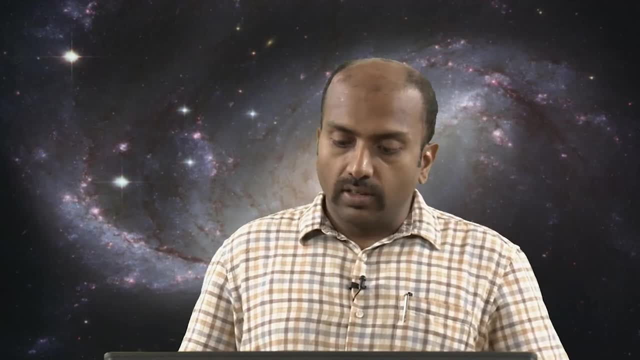 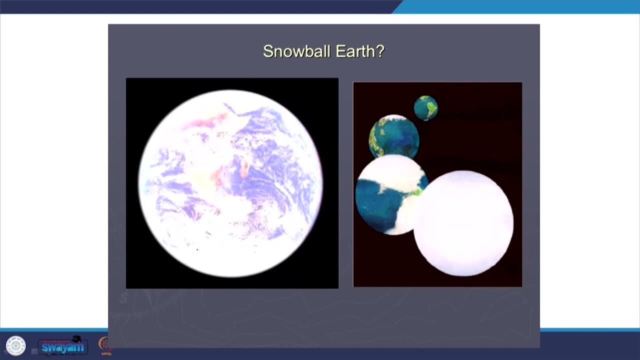 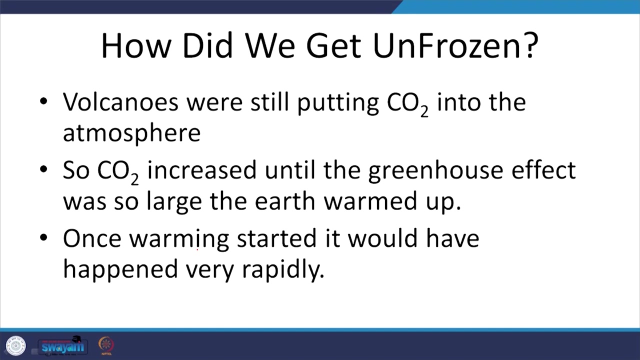 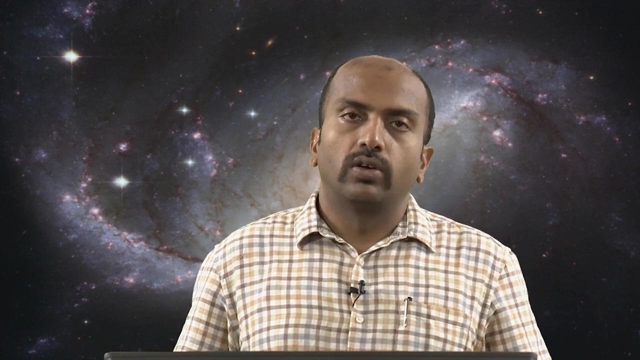 feedback which could have resulted. but So this is, I mean, an artistic impression, where the Earth must have turned into a snow, or let us say, glaciated Earth, with the decreasing levels of CO2, which is definitely a possibility Now, but we did not. we did not completely get a nice ball, or let us say snowball. 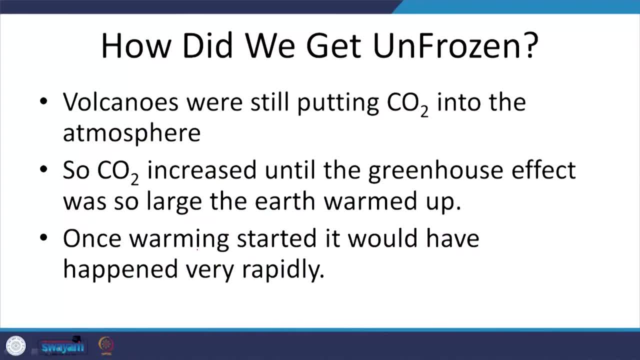 what happened is there were still volcanic eruptions which were active that time. there were still a lot of volcanic eruptions were still throwing a lot of water vapor and a lot of carbon dioxide into the atmosphere. So this CO2, was increasing at the same time with the time, at the same time as it happened. 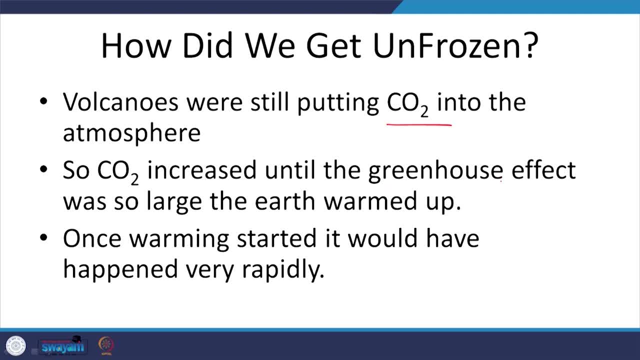 So CO2 increased until the greenhouse effect was so large that the Earth warmed up and it got out of the ice age. So once warming has started, it would have happened very rapidly. So that must have gotten us out of the ice age Now in the last 500 million years. So 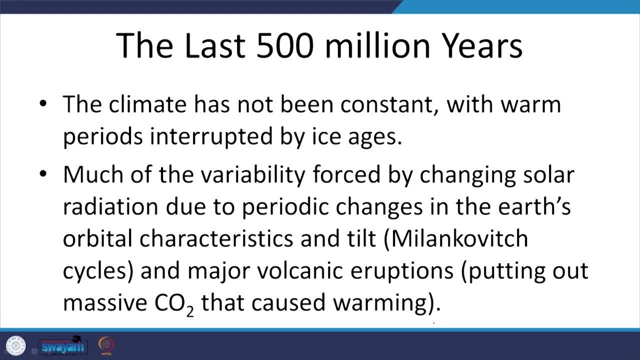 the climate has not been constant, with warm periods interpreted by ice ages. So there that the average temperature is what I am talking about. So warm period is some point of time where the average temperatures have gone up and ice age is the period of time when the average temperatures have gone below. 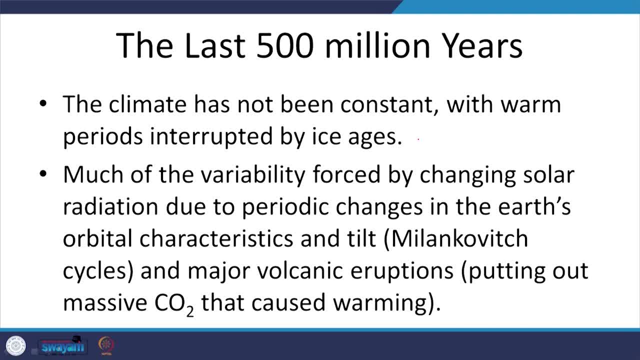 the limit. So much of the variability was forced by changing this solar radiation due to the periodic changes in the Earth's orbital characteristics and tilt. These cycles are called as Milankovitch cycles, and major volcanic eruptions were trying to put as much as CO2. 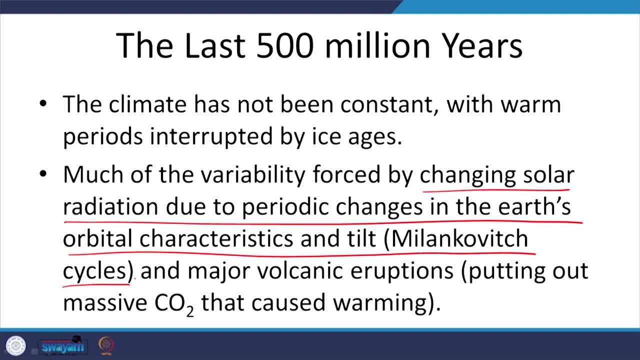 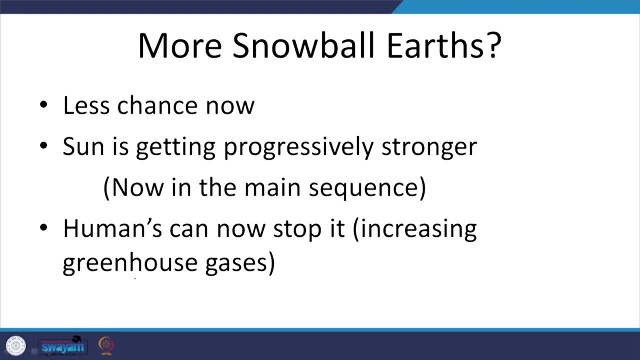 possible into the atmosphere just as much as possible, Just to make sure the temperature fall beyond the certain limit. ok, So there is a chance- I mean, there are very little chances, of course- So we can find ice ages in the coming future. 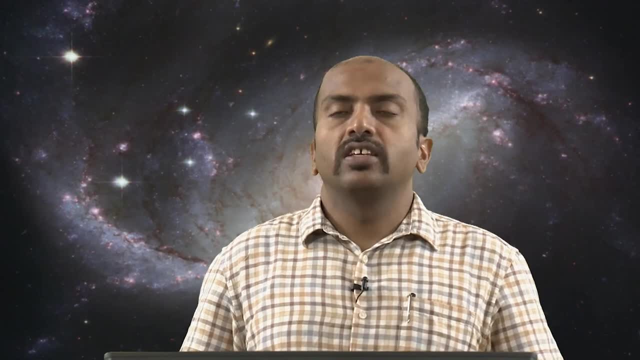 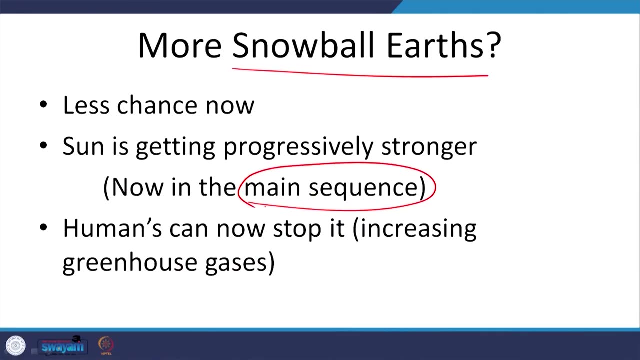 And the main reason is that the sun is getting stronger and now it is a main sequence star. you know that right So now, even the anthropogenic effects, such as increasing the levels of CO2, can avoid the formation of or the resulting of snowball earths. So this is the average temperature variation over very long amount. 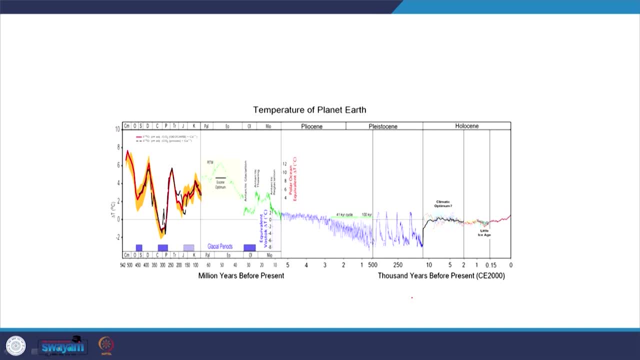 of time, a large amount of time. So what you see is there have been severe warmings and there have been severe coolings. So now this average temperature is what you see here, and if this average temperature goes beyond a limit, you call. 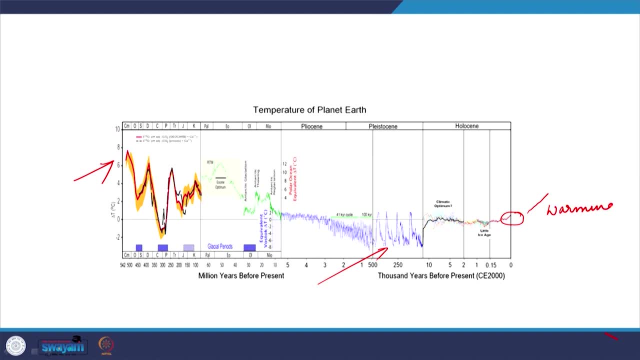 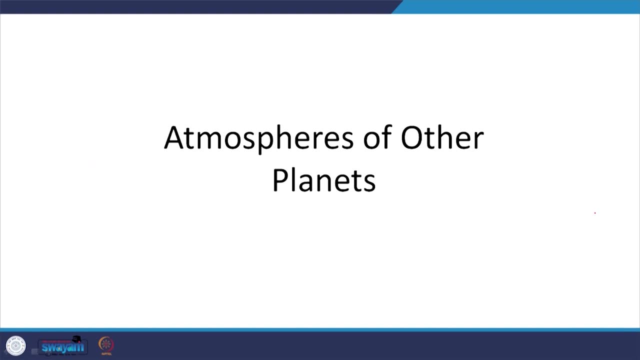 this as warming. There are several reasons for this. I mean, this is a very elaborate discussion in itself. So here, what you can see is so this is what happened, which, in its entirety, has resulted in the formation of the earth's atmosphere to the composition that we know today. So just before we go ahead, we will make a recap. So the recap is that the earth's atmosphere was resulted mainly from the volcanic eruptions. So volcanic eruptions gave away a lot of water vapor into the atmosphere. This water vapor was broken or dissolved. 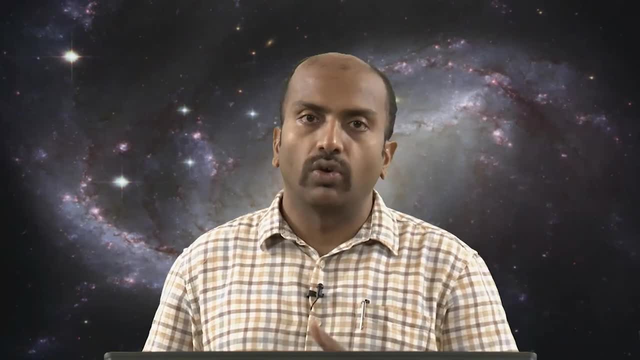 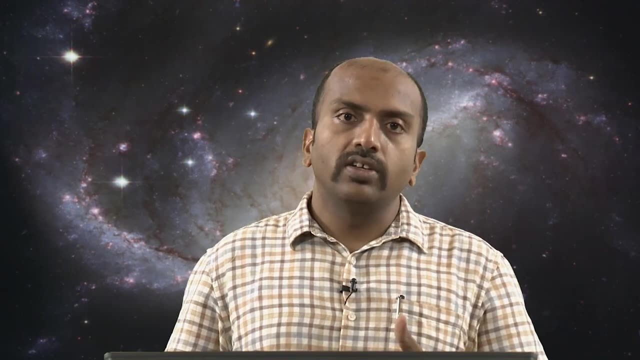 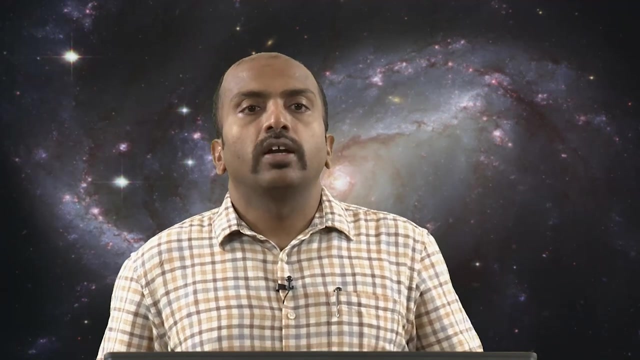 by the ultraviolet radiation, giving you the initial hints of oxygen, and later a certain other reaction, which is called as the photosynthesis reaction, took over and this reaction, being fast, gave away or created a lot of oxygen in the atmosphere. right, The nitrogen levels were almost the same since the beginning. they since the nitrogen since 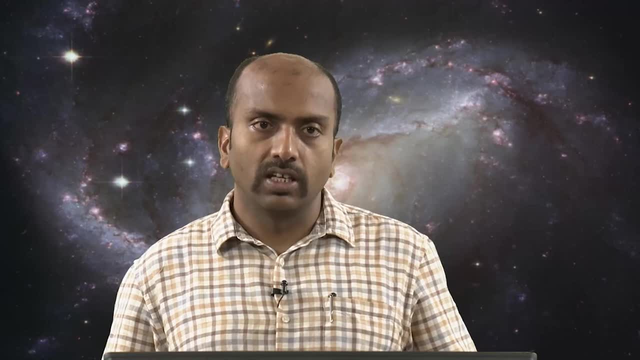 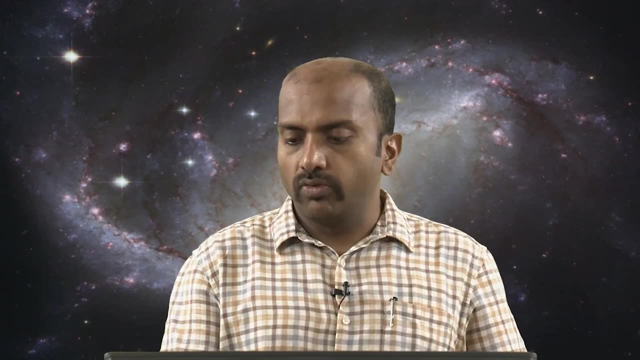 nitrogen is inert, chemically inert, it would not participate much in the chemical reactions with the other species in the atmosphere. So it remained as it is and today, in today's chemical composition, the earth's atmosphere is always to be remembered as 78 percent nitrogen and 21 percent. 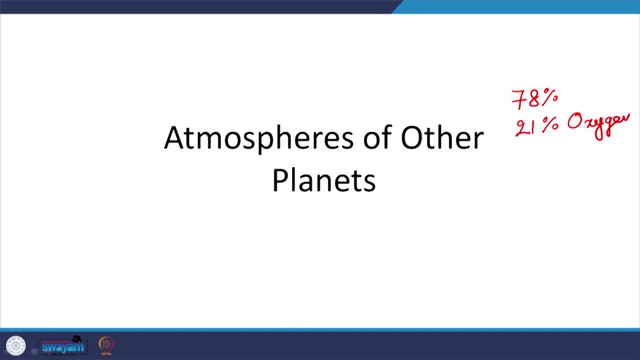 oxygen, right. So this is the chemical composition which we know is very much suitable for the existence of life on this planet. So this is a very important thing. So this is what makes the earth livable or habitable, right The beginning. we know that the planet earth has formed by the agglomeration of large sized 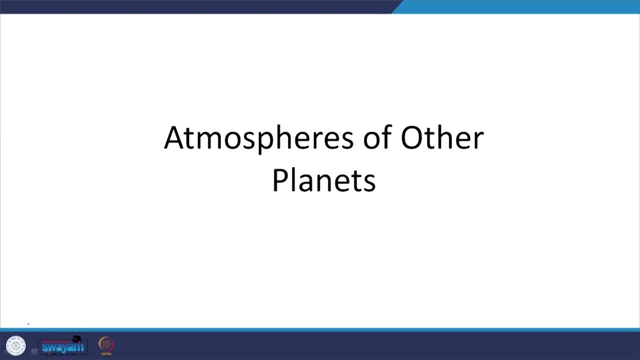 objects which are called as planetoids. They came together. there was a volatile substance which was trapped in between these rocks and as the gravity grew stronger, these pieces came together and there was a lot of compression between these pieces and there huge temperature increase in this system and all the heavier elements sank to the deep or 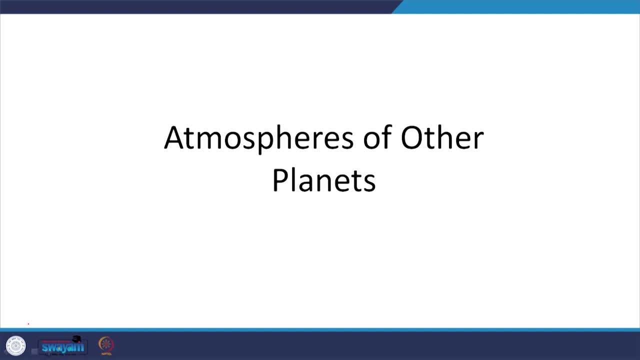 they occupy what is called as the core, and all the lighter elements were raised to the top right. So this is what happened. I mean right Now there is a very strong reason for us to believe that, since the entire system, the solar system itself, resulted out of the nebula of gases and dust. So 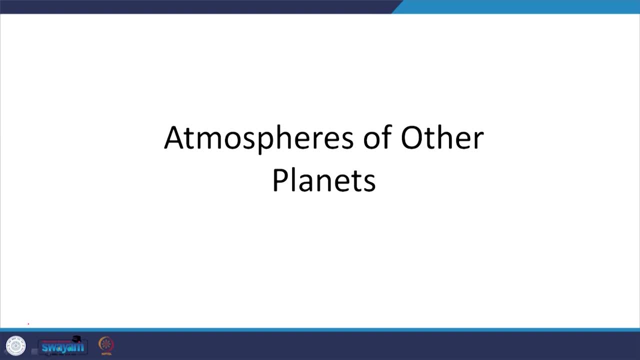 every planet that has formed must have formed at the same time as the earth and must have gone through the same physical or chemical processes which have resulted into the formation of earth or the earth's atmosphere. right Now. we know it now very well that earth's atmosphere is the only 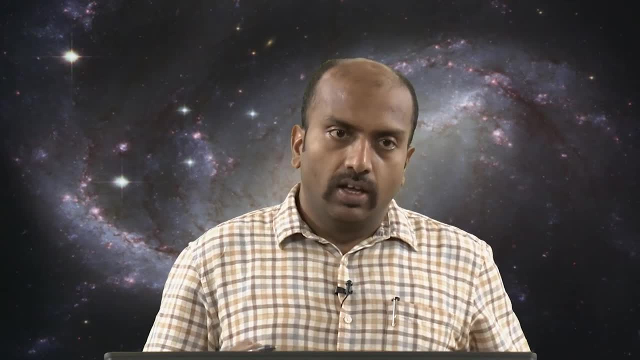 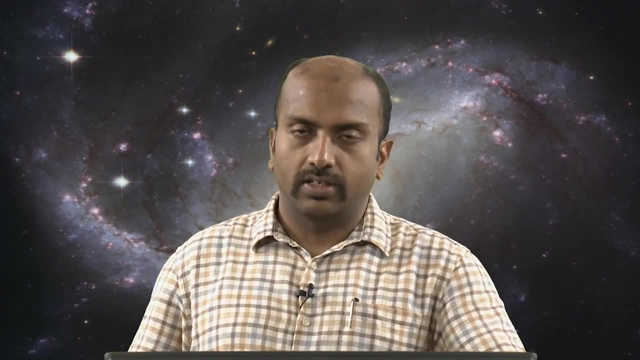 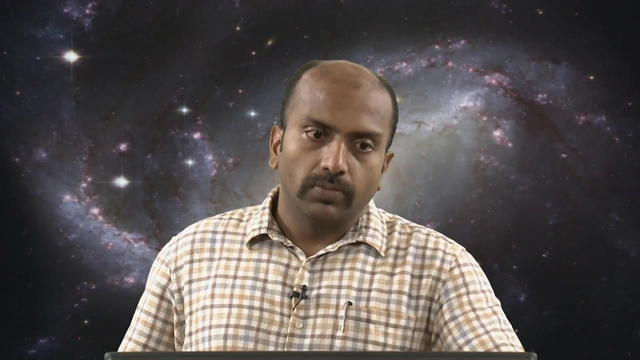 place which supports the existence of life. Apart from life, earth's atmosphere is also very different or has a very clear contrast with respect to the earth's atmosphere of earth. So we will see how it is different right Now. it may be interesting to find out what were the 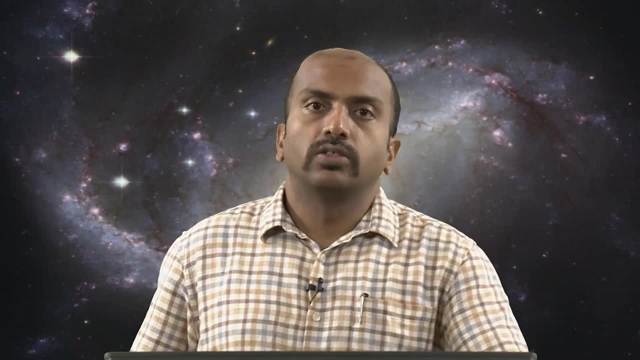 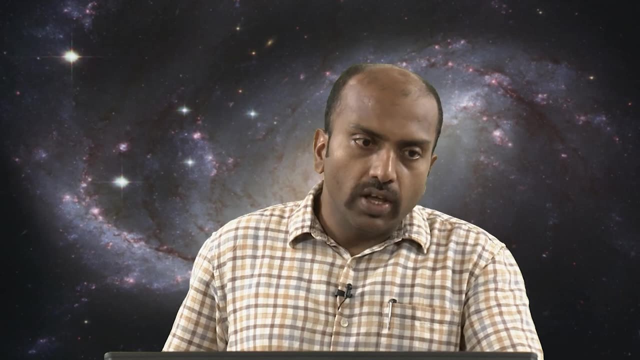 processes which went different in other planets, So that now you have a different chemical composition on those planets, right, but that is a discussion in itself, right? So today, what we will do is we will not go into the details as such, how or why this composition has resulted. 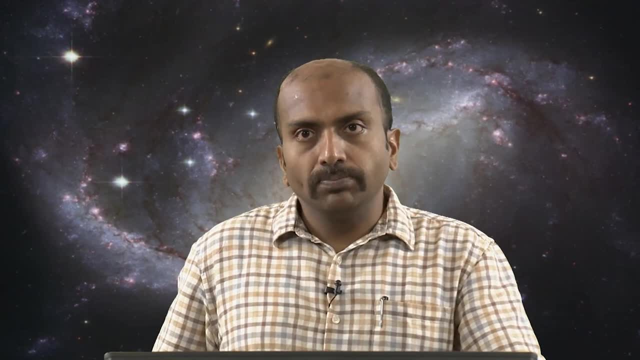 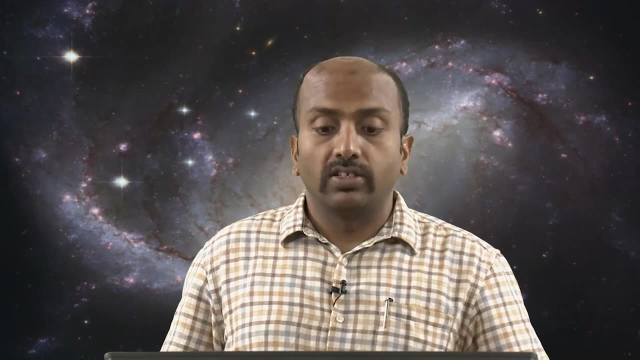 in on these planets, but rather what we will do is: we will see what is the, what are the different features of atmospheres of other planets in our solar system. ok, Now, to begin with, let us say: the planets in our solar system are mainly categorized into: 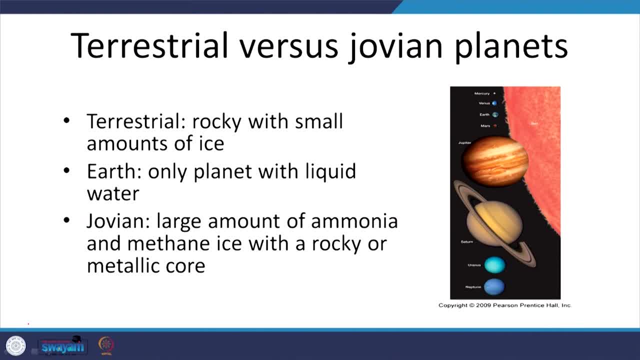 two different types: One terrestrial planets and another jovial planets. Jovian planets are the ones which have, which have no rocky surface, which are basically gas genes, and terrestrial planets are the ones which have rocky surfaces. Let us say that means a surface where you can put 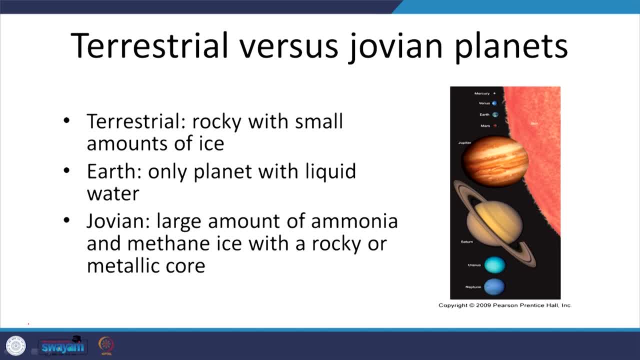 your feet on, So it is a surface where you can put your feet on Or a surface where you can land. ok, So terrestrial planets are the ones which have rocky surfaces and jovian planets are the ones which does not have a rocky surface. ok, 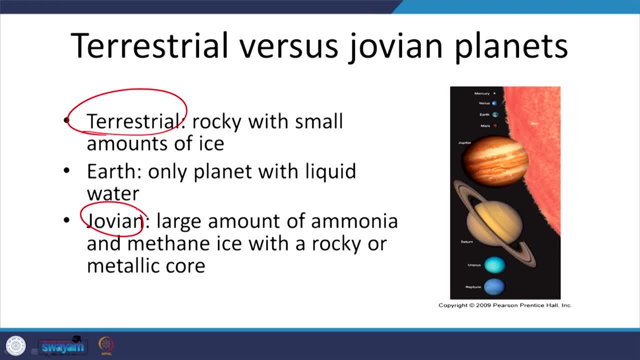 So terrestrial planets generally have some small amounts of ice, of course, and earth is the only planet with liquid water as of now that we know today. There are other planets or there are other moons where water is has proven to be present, but that is a. 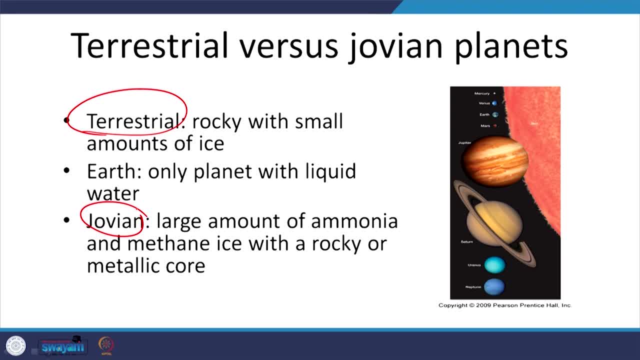 question away. right, And jovian planets are mainly characterized by large amounts of ammonia and methane ice with rocky or metallic core. Generally, the first four planets- Mercury, Venus, Earth and Mars- are terrestrial and the rest are jovian. Now, these planets, let us say, for example, some of them. 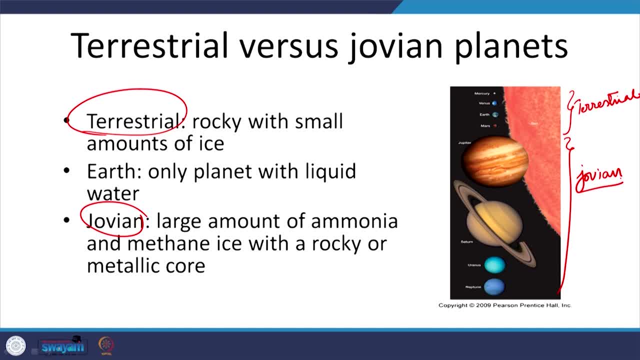 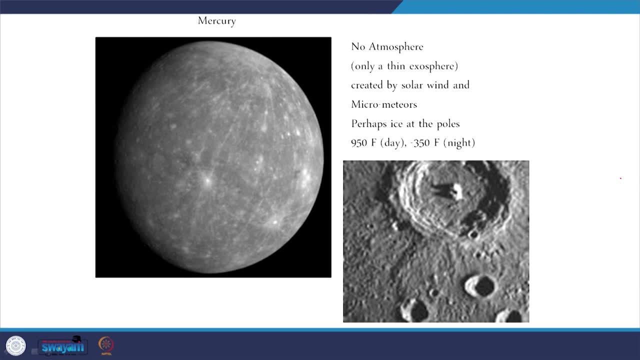 have not rocky surfaces, but they have ice sheets. I mean, they are frozen. So the entire planet itself is an ice of not liquid or not water. rather, it is an ice of gas. ok, That is a different thing. right Now, let us see one by one. ok, Now let us start with Mercury. 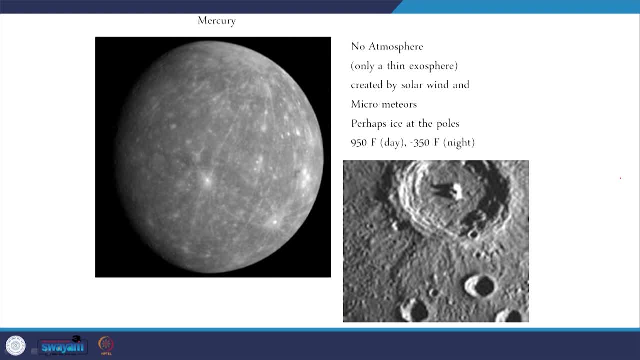 Mercury practically has no atmosphere, only it has, it exists, only it exists. it has only a thin exosphere which is mainly created by solar wind and micrometeors. ok, Now, there were some reports which predicted the formation or existence of ice at the poles, not confirmed anyway. 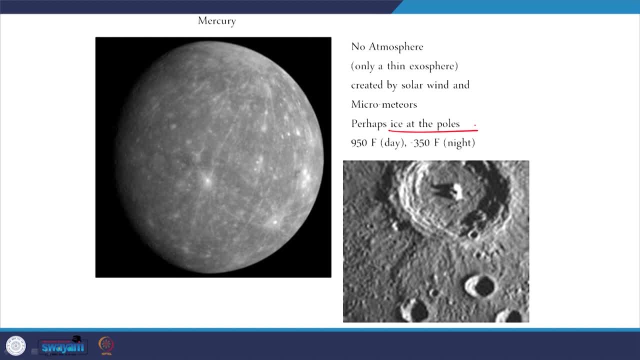 The important feature about Mercury is that Mercury's average temperatures fluctuates a lot because of the lack of atmosphere. that is why- So we have already seen- because if you do not have an atmosphere, or if you do not have CO2, then your, the planet will lose heat easily. 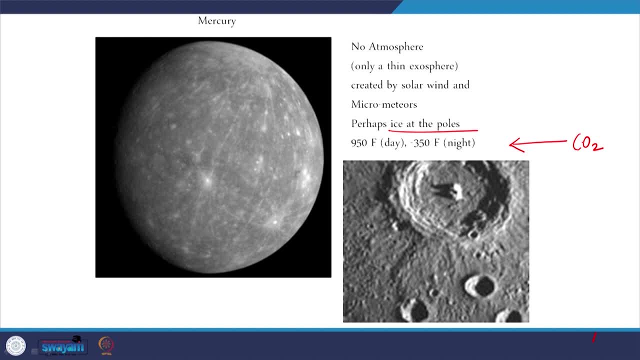 and will gain heat easily. That means that is why the temperatures on Mercury vary a lot. So Mercury is the closest planet to earth- sorry, closest planet to the sun. of course, it receives immense amount of energy in terms of radiation, or particle flux, from the sun, So sun basically cooks up the entire planet when it is in the day, and when it is the night, there is, since there is no source of energy. So sun, the Mercury, immediately loses the heat, and then the night time, temperatures reach a very low value of nearly minus 350 Fahrenheit. ok, Now then you have 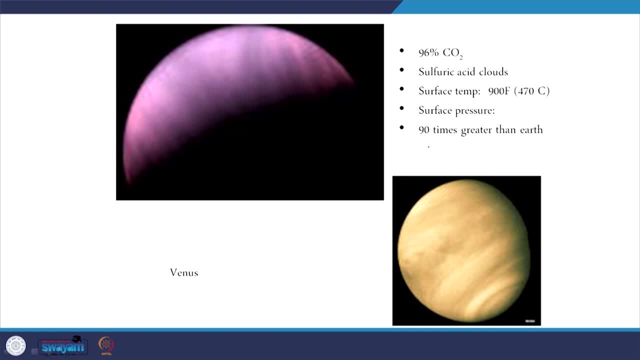 Venus. Venus is to our, the our neighbor, So which has 96 percent of CO2. So this is the mainly CO2 dominated atmosphere. I mean, it is mainly nothing else actually. So Venus also has sulfuric acid clouds. Venus has very important phenomena which are not totally understood. It has 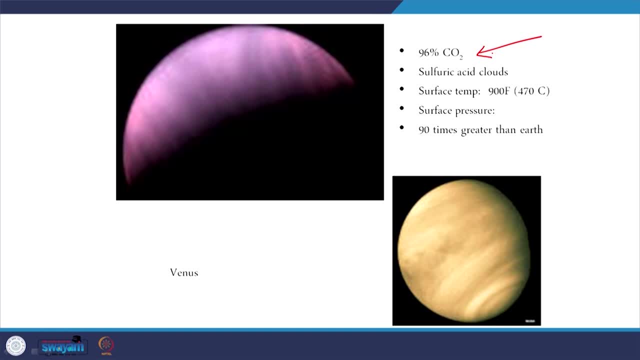 sulfuric acid clouds suspended in the atmosphere. its surface temperature goes nearly as high as 900 Fahrenheit and it has a very high surface pressure. So this is an interesting phenomena in which happens in the Venus. Venus surface pressure is immensely high, which is nearly 90. 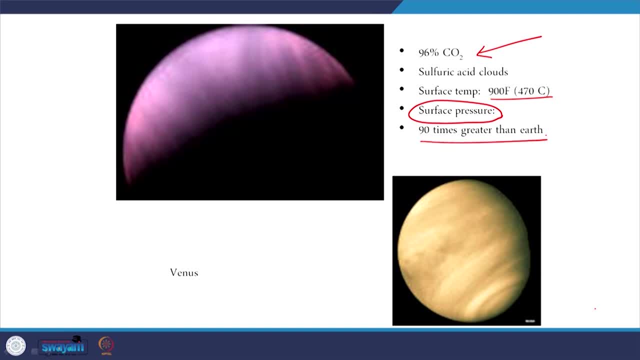 times more than that of the earth. ok, So which is a very big number in itself. ok, Now why is it that Venus surface temperatures are very high is mainly because of the large amounts of CO2. CO2- you know, you have seen that CO2 tends to. 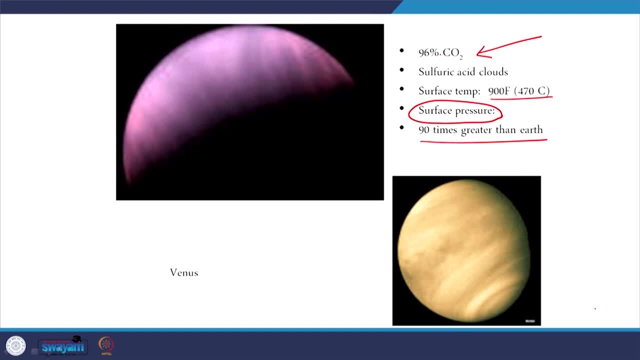 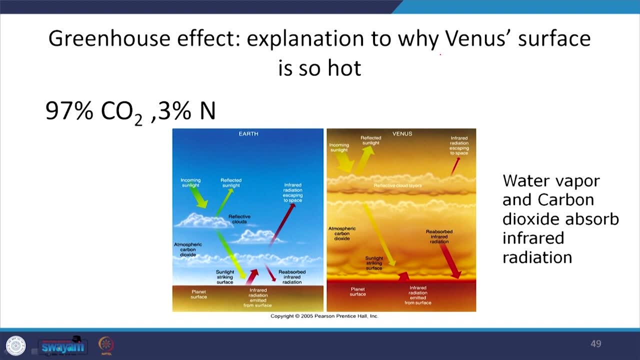 trap heat and it would not allow heat to be given away from the planet. right, we have seen that. So, because? so this is basically the an example of greenhouse effect, where you see this, the figure on your left is the earth and this is Venus. So what you see, due to the enhanced availability of 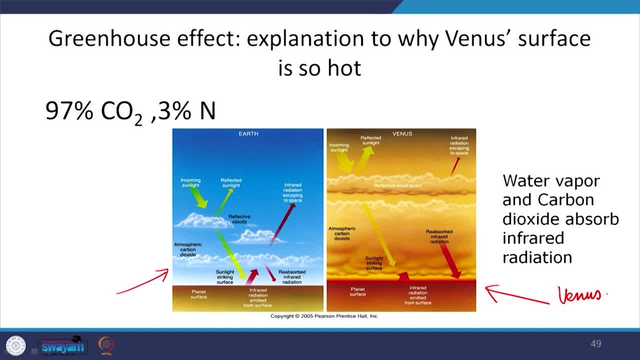 CO2 to a very large extent the greenhouse effect is enhanced. I mean, it is an enhanced greenhouse effect which basically traps the outgoing radiation and it would not allow the outgoing radiation to escape into the space and it will heat the planet to a very large 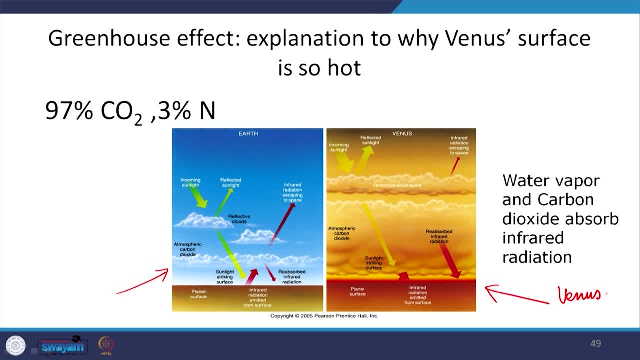 temperature. So the point is, the Venus is not at a particular distance where this surface temperature is 900, where its surface temperatures should be 900 Kelvin, but it is because of the large availability of carbon dioxide, which has the ability to trap the heat. This is just a figure. 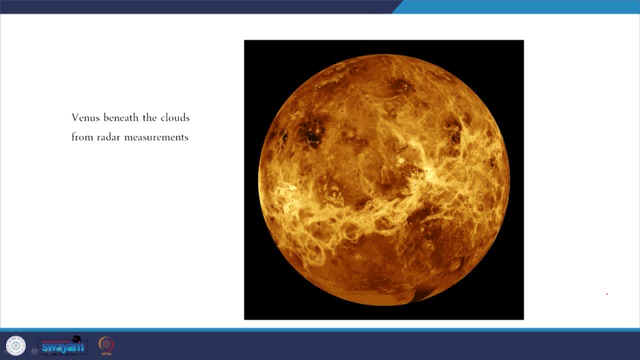 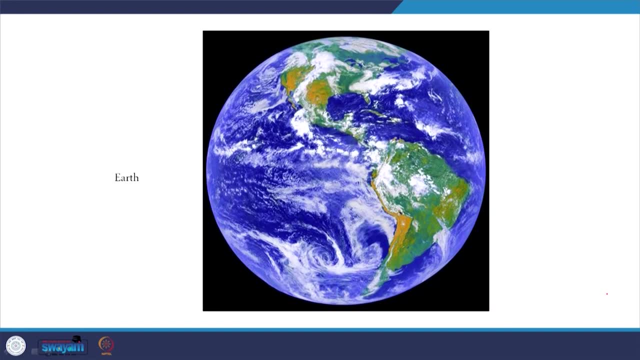 of this Venus beneath the clouds, from the radar measurements. So you see several patterns on this on this planet. right, Then you have the earth. of course, we know the chemical composition of earth and how it has evolved, how it has come to existence today the way it is. we know several. 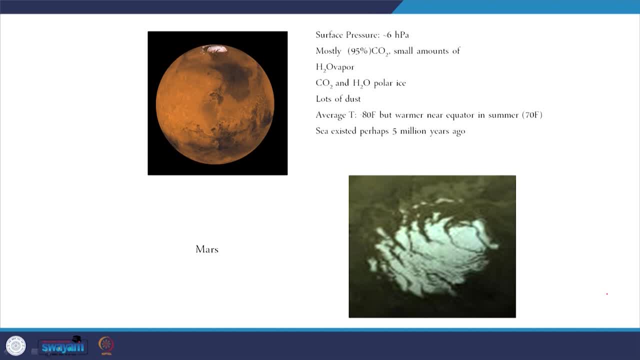 other features about the earth's atmosphere itself. right. Then you have on the right: the nearest neighbor is Mars, which is which has: the surface pressure of Mars is nearly 6 hectopascal and the atmosphere is 95 percent is CO2 and small amounts of water vapor, And it has also. 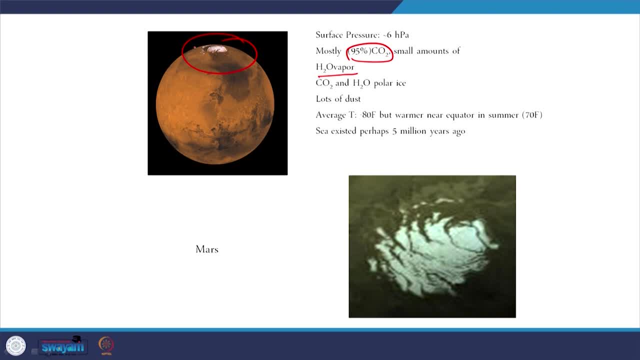 been seen that in the poles, Mars has the ice formation, ice crystals made up of carbon dioxide and water vapor. Mars, of course, has a lot of dust, I mean it has a rocky surface. The average temperature is minus 80 Fahrenheit, but it is generally warmer in the near the equator. 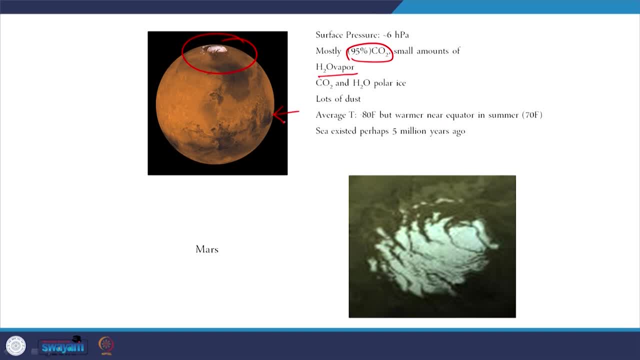 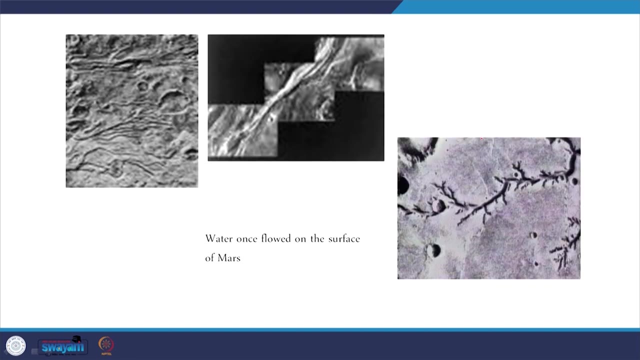 in the summers. So that means the temperature of the pole at the equator is not as high as low as minus 80 degree Fahrenheit. And it is believed that their water bodies must have existed on the surface of Mars nearly 5 million years ago. So this is still unverified, ok. 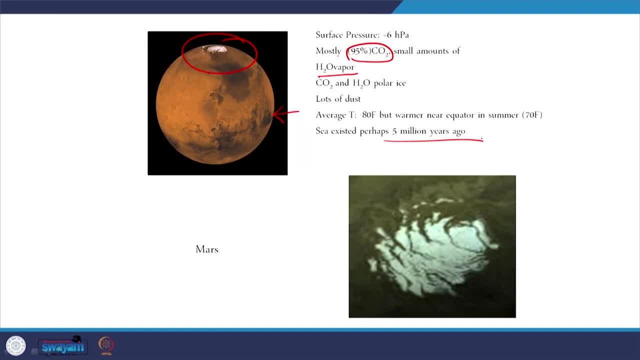 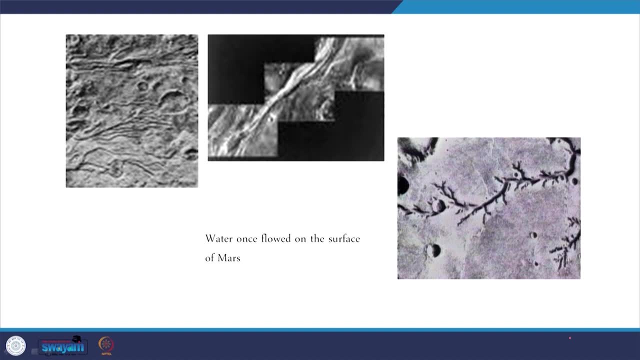 So what you a very important or very prominent feature that you see on the Mars. if you see, if you open any image of Mars, you will always be able to see that there were a lot of, there are a lot of patterns in which which indicate that the temperature of the equator is not as high as 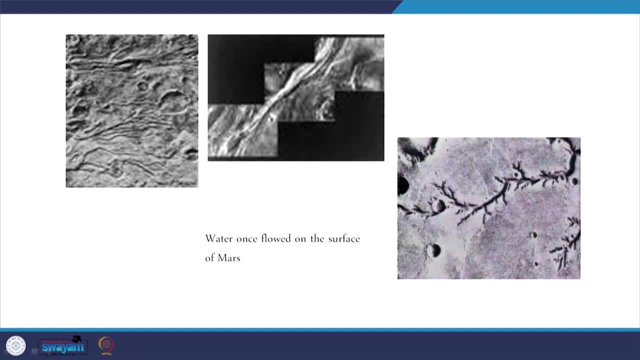 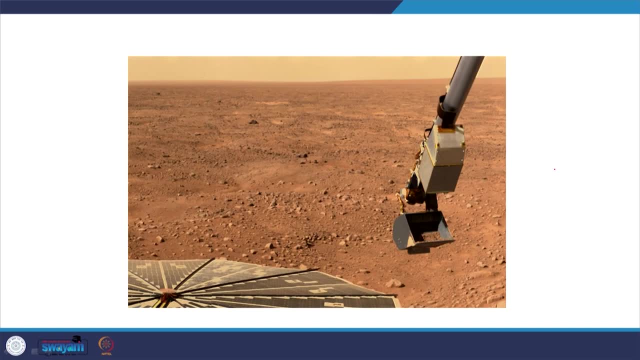 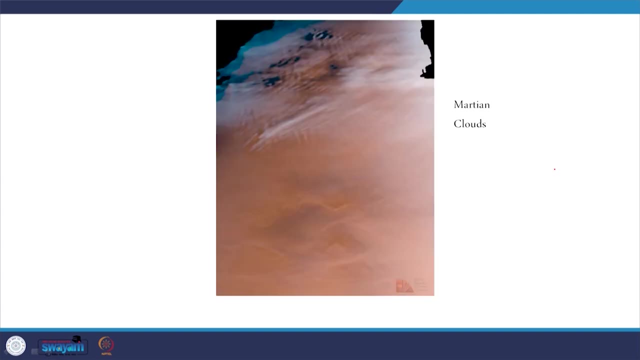 indicated that water must have flowed or there was water flow on the surface of the planet the several million years of million years ago. So this is how it looks like. the Martian surface looks like the red planet, right So, and the Martian clouds have also been. 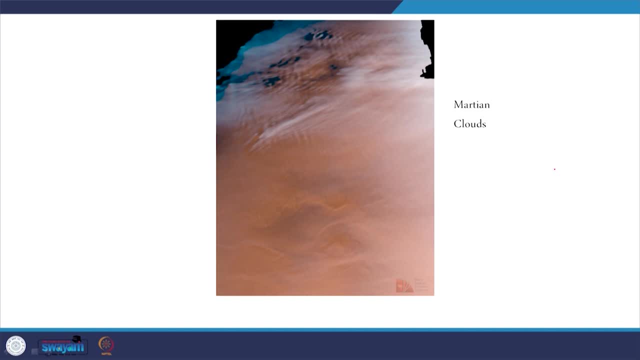 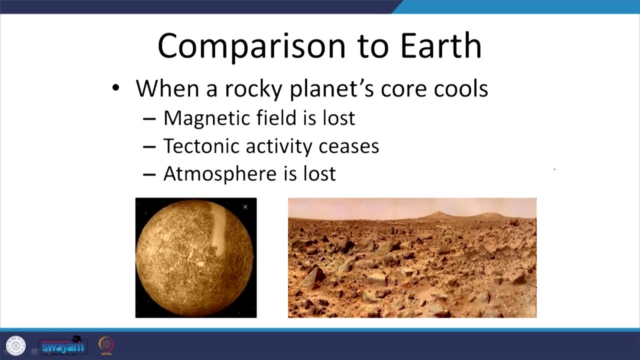 seen by several space crafts right Now, when you compare the Martian surface or atmosphere, what generally happens is when a rocky planets core cools. I mean now we know that the earth's core is the molten iron core that we have. the center of the planet is a very hot. it is molten. 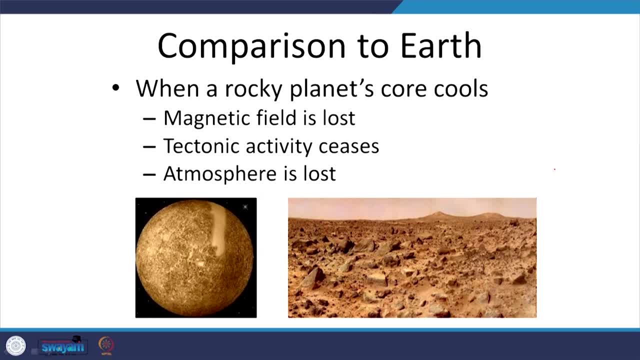 So it indicates it is very hot. it is rotating right Now when this core loses its heat. the core can lose heat due to a lot of reasons, due to many reasons. What immediately happens is, if the core loses heat, the magnetic field is not going to be able to rotate. Now, if the magnetic field is not, 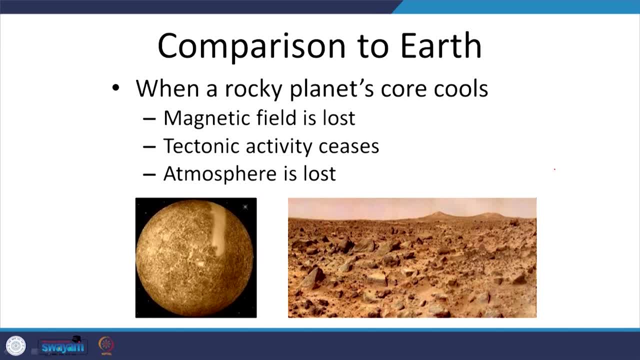 going to be able to rotate. the magnetic field that it generates is mainly lost. So you lose the dynamo right and the tectonic activity which moves the surface in and out. Basically, the earth surface actually turns around. we know that. I mean it happens over several millions of years. 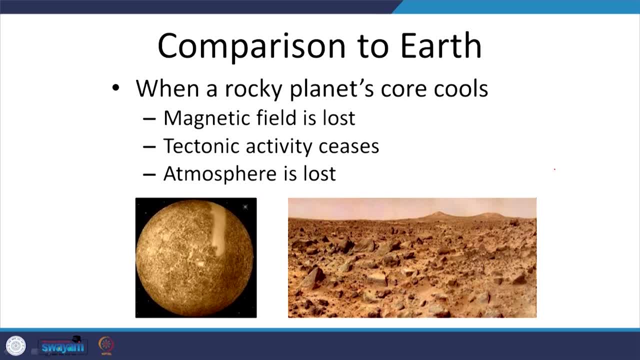 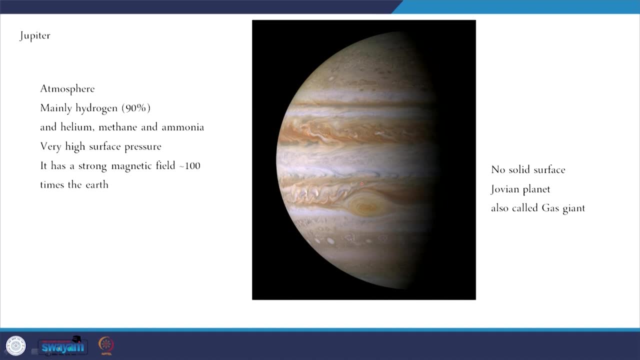 it takes several millions of years, but earth's surface eventually turns out. So the tectonic activity lose, ceases to exist, and then you have: the atmosphere is lost. That is what must have happened to these planets, right? and then you have Jupiter. Jupiter is the. 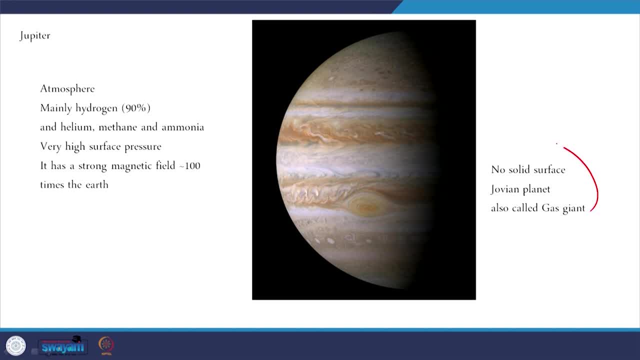 gas giant. I mean that means there is no surface, there is no solid surface to land or to stand, let us say, and which is a jovian planet by our definition right, and it is also called as a gas giant. Jupiter is a very large planet, So atmosphere of Jupiter is mainly 90 percent. 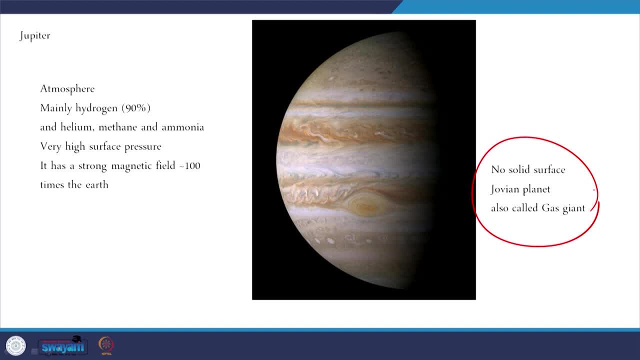 hydrogen and the remaining is helium, methane and ammonia. So these are present in a very, very large numbers. So this also has a very high surface pressure. it has strong magnetic field. The Jupiter has a very strong magnetic field which is nearly 100 times the earth. 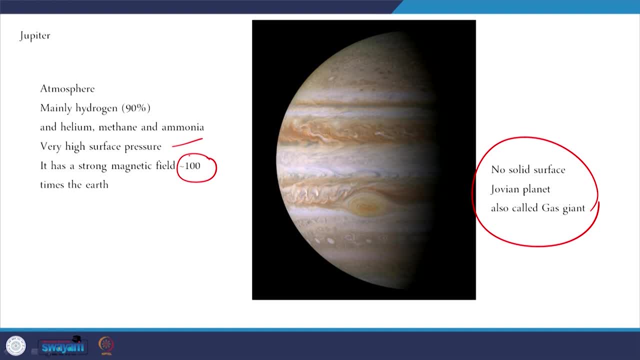 You know, in our discussions, you know in the entire course, two things really matter to us. what are they? One: we will be interested to understand processes about atmosphere. When we say atmosphere, we generally are referring to the processes which are mainly dealing with neutral constituents. Then you have another processes. 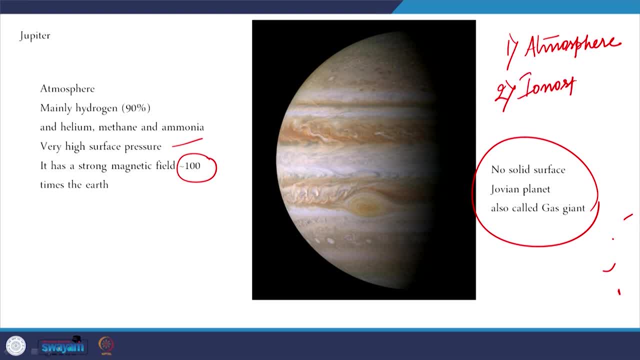 another set of processes which are different, which we generally call as ionosphere right? So in this, the in the second topic, we will mainly discuss about the plasma processes. How so this is? these are the processes in which you talk about magnetic fields. 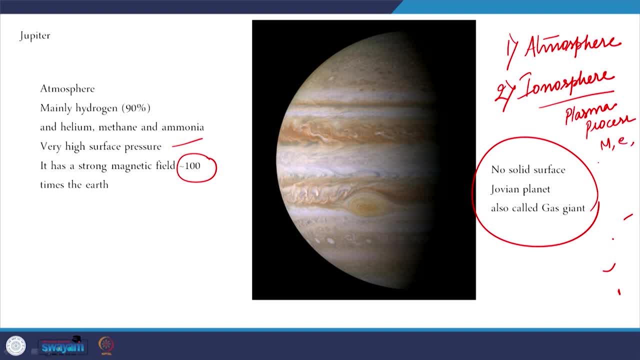 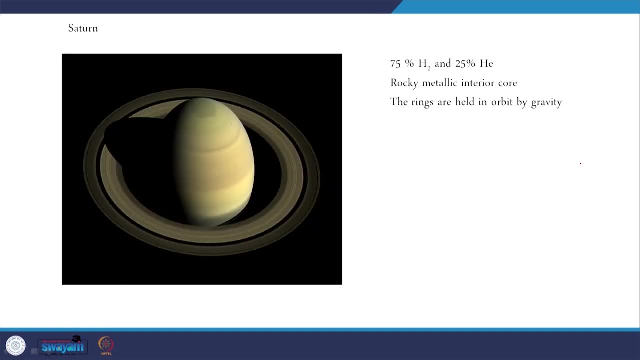 you talk about charges, you talk about electrons, you talk about, you talk about plasma, right? So for those discussions, probably the strength of magnetic field, or the origin of magnetic field, or the shape of magnetic field, these things will be relevant. ok, So then the next planet is Saturn. Saturn is mainly 75 percent hydrogen and 25 percent helium. 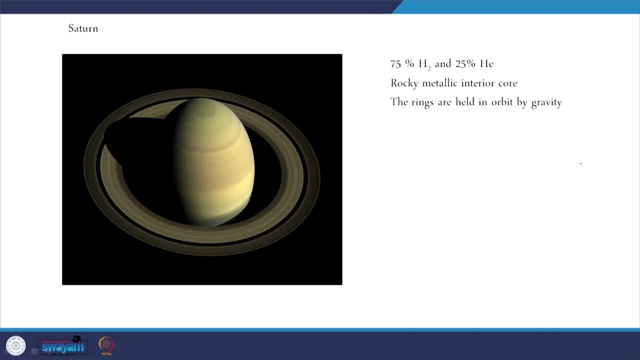 So Saturn is also hydrogen and helium. This composition is not so different from the composition of sun itself. We have already seen that. So that is, sun is also a similar chemical composition, but the only difference is their sun has as a reactor which fuses hydrogen to form. 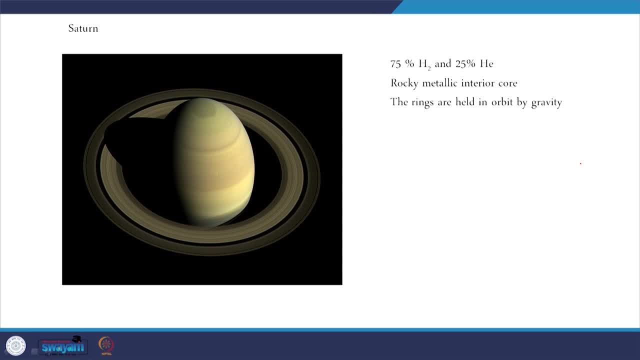 helium right. the other planets do not have it. This planet is believed to have a rocky metallic interior core. It is the core, not the surface, that I am talking about, and the rings that you see, which nearly span over nearly 18000 kilometers, are basically held to the planet: the. 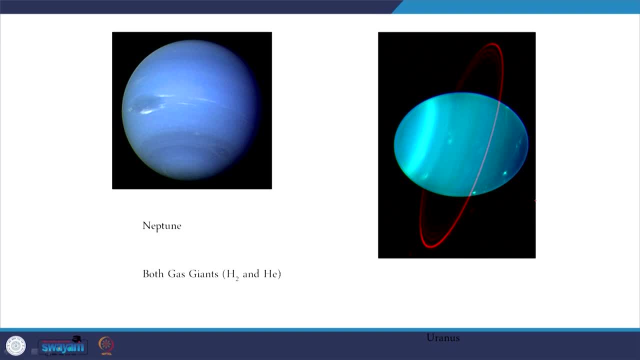 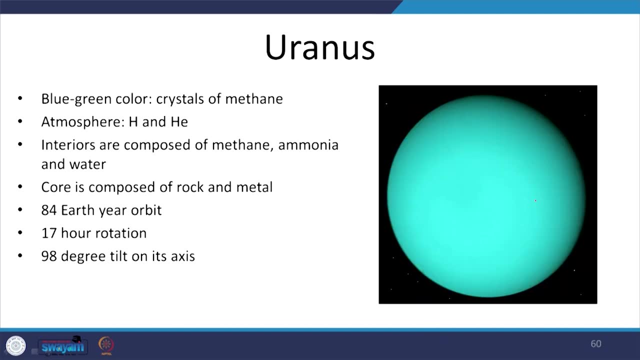 Saturn by its gravity, And you have another two gas genes which are Neptune and sorry, Uranus and Neptune. Both of these are gas genes. let us say Uranus, let us say, which appears in blue green color. bluish green color is due to the crystals of methane that exist on the planet and the 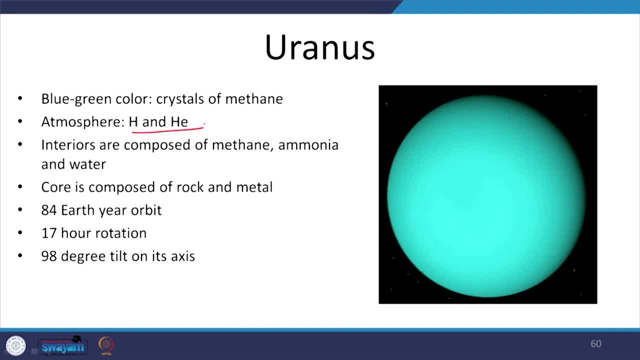 atmosphere is mainly hydrogen and helium, again So, and interior is composed of methane and ammonia water. So we do not know what exists inside the ice- I mean icy surface, and the core is composed of rock and metal. It is a. I mean these two are the rotational characteristics of the planet that 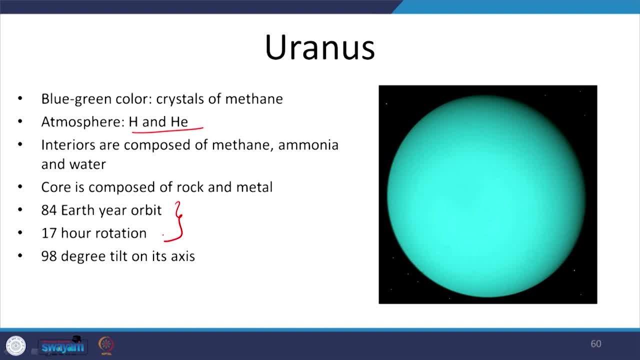 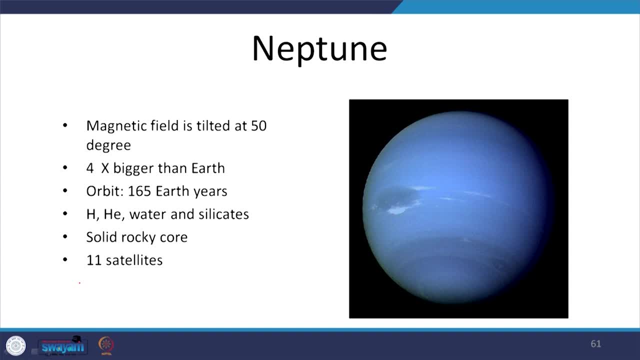 means it takes a very large amount of time to rotate around the earth and it has a huge tilt of nearly 98 degrees on its axis. And Neptune, the farthest planet in our solar system, it has a magnetic field, is tilted at 50 degrees and the atmosphere is mainly hydrogen and helium.